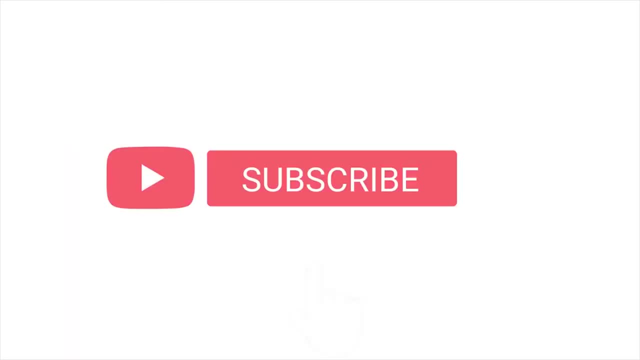 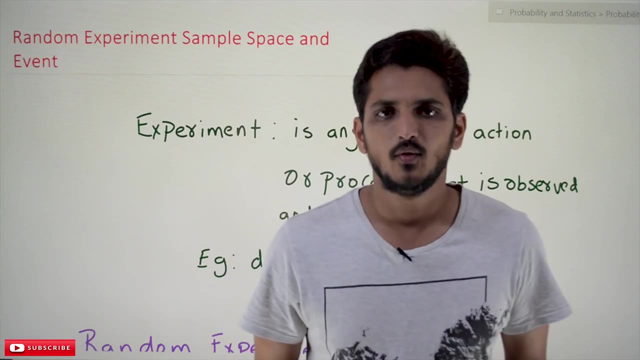 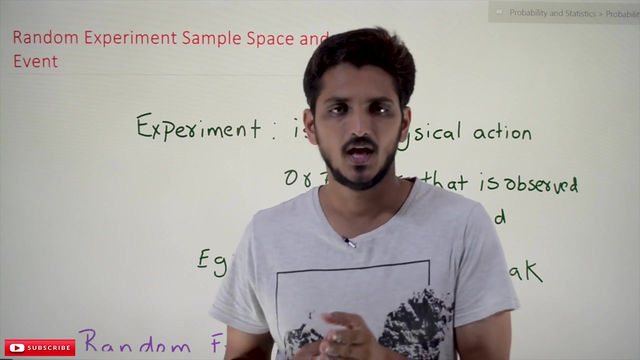 Hi, welcome to Learning Monkey. I am Raghu here. In this class we will discuss about random experiment sample, space and event. We will understand the definitions. In our last class we clearly discussed about what probability means and what is biased and unbiased. 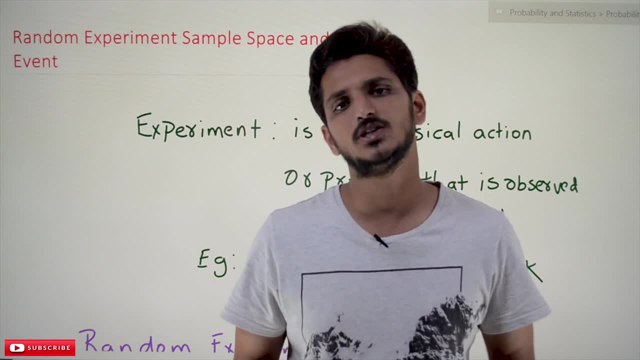 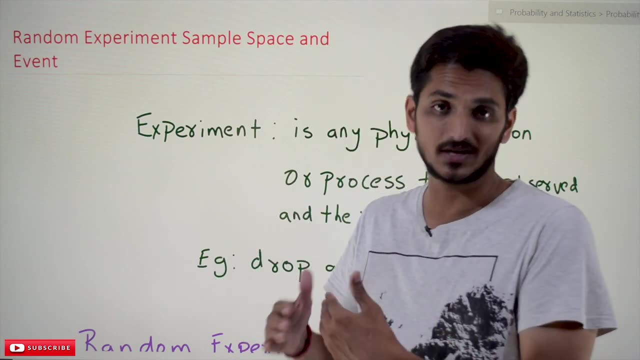 Please watch that class and come back here. The link for the playlist is provided in the description below. The definitions which we are going to discuss here in this class will help you a lot in understanding our next classes, where we are going to discuss about how we find the probability values and all those things. 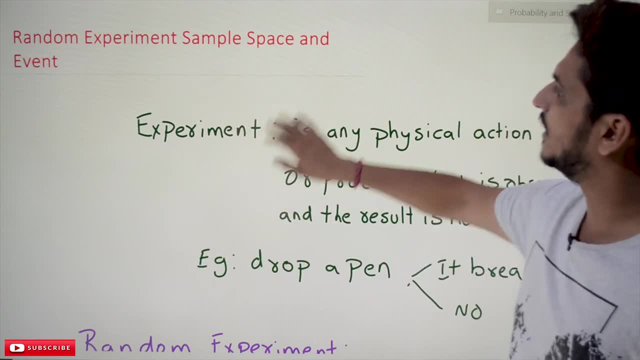 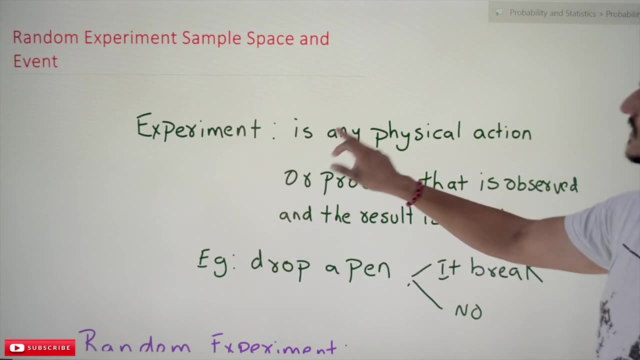 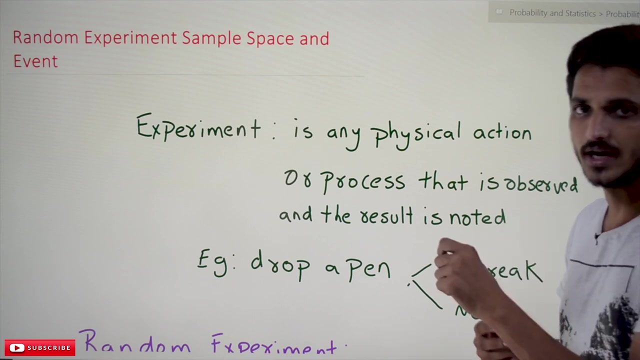 Coming to the definitions random experiment. Before going to understand what random experiment means, first we will understand what experiment means. Experiment means it is a physical action of process that is observed and the result is noted. You do any physical action or a process, that process is observed and the result is noted. That is what experiment means. 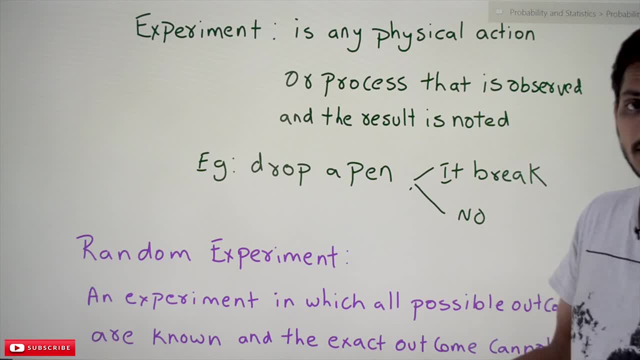 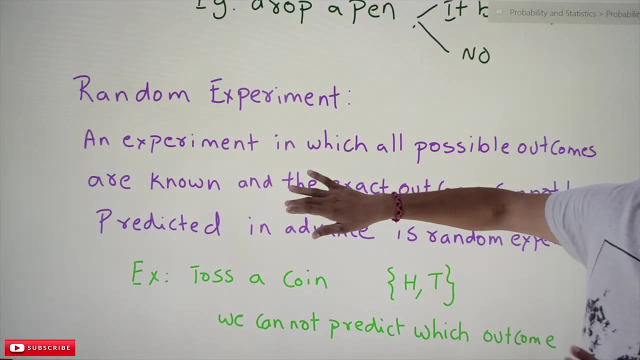 Example: drop a pen. It is an experiment. It may break or it may not break. So that is the output you are taking a note of. So this is an experiment. Now coming to the next definition: random experiment means. So it is little confusion to understand. 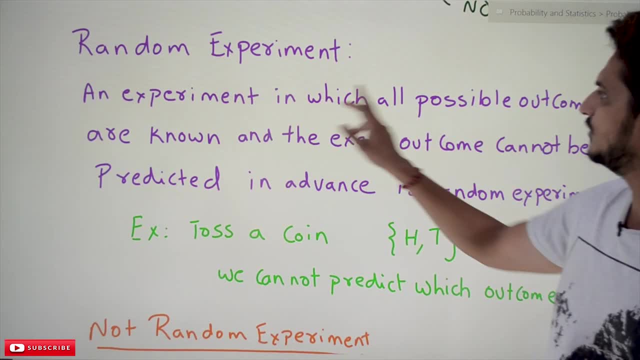 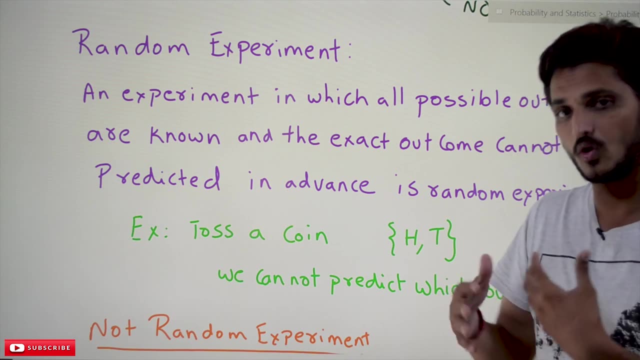 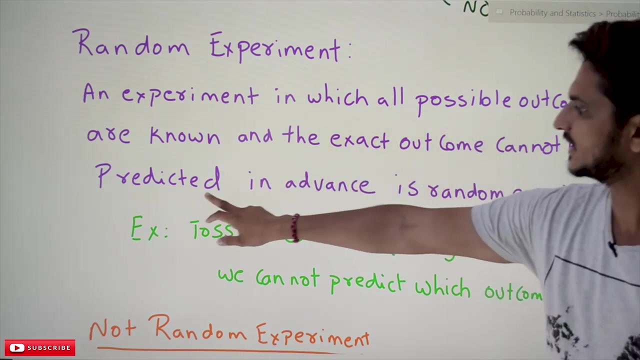 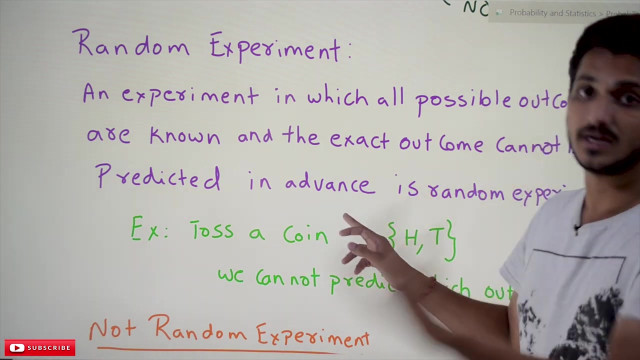 So watch carefully An experiment in which all possible outcomes are known, We know when we do the experiment, we know what outcomes it is going to get, And the exact outcome cannot be predicted in advance. That is what random experiment means: The exact output cannot be predicted in advance. 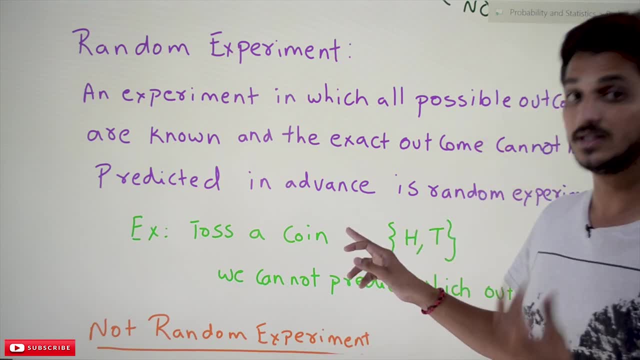 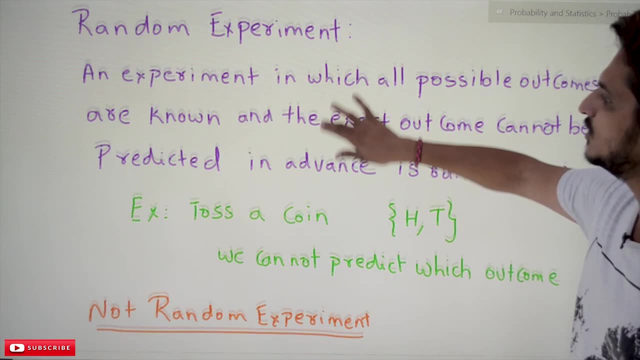 We know all the possible outcomes, But the exact outcome cannot be predicted in advance. That is what random experiment means. Anyhow, with example, you are going to understand better If you toss a coin, what is the possible outcomes that you are going to get. 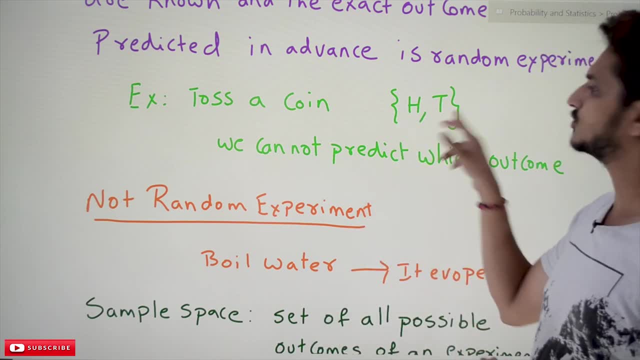 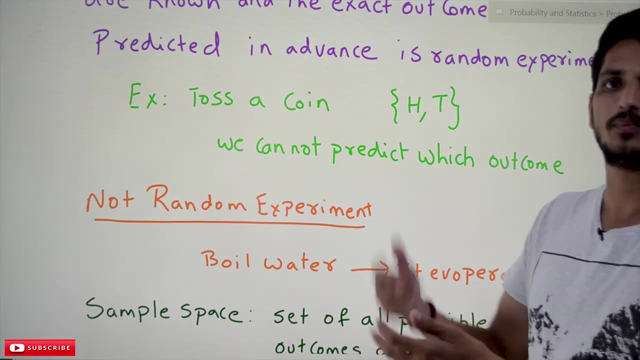 When you toss a coin. it may show up head, it may show up tail, But what is the exact output that it is going to come? We don't know. It may show up head, it may show up tail. These are the possible outcomes. 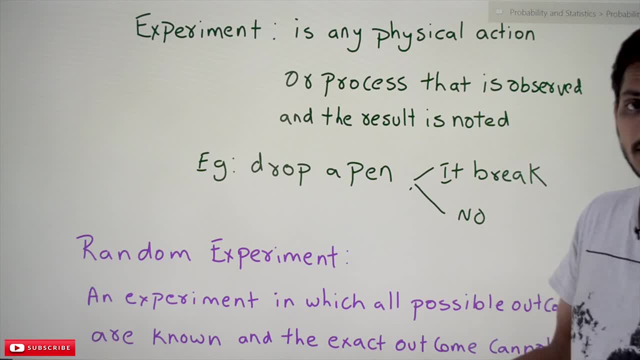 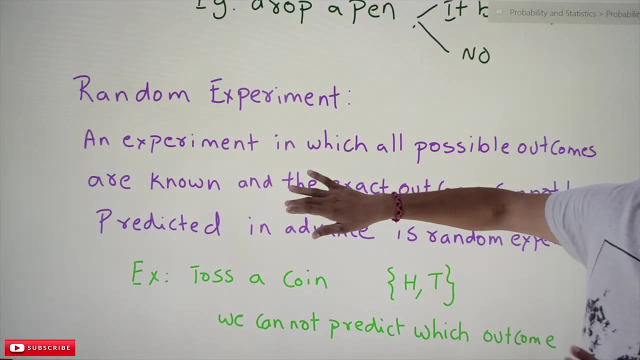 Example: drop a pen. It is an experiment. It may break or it may not break. So that is the output you are taking a note of. So this is an experiment. Now coming to the next definition: random experiment means. So it is little confusion to understand. 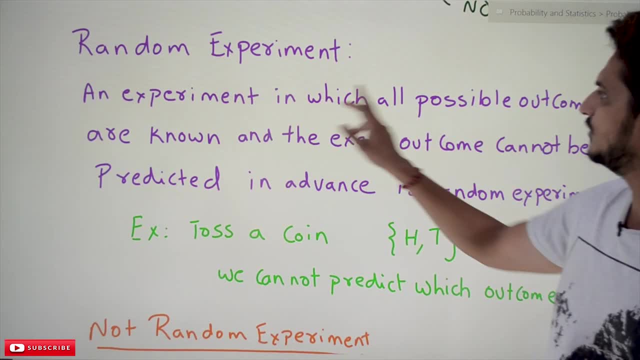 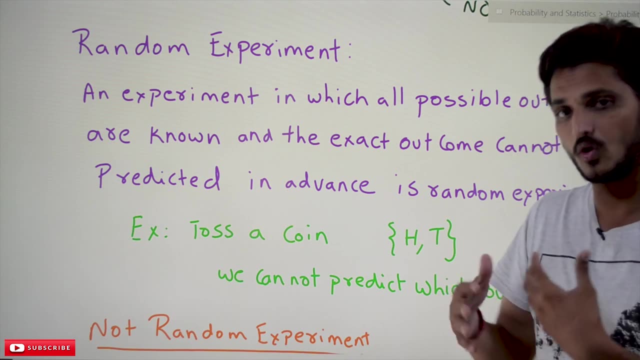 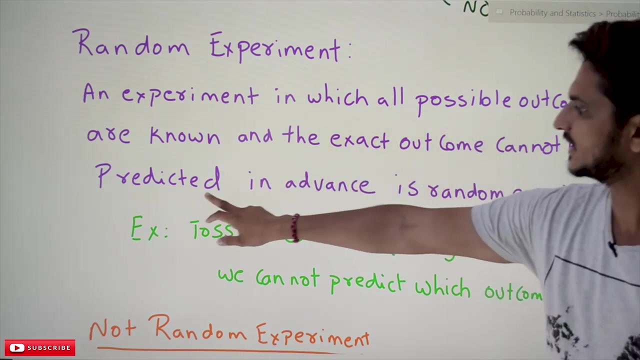 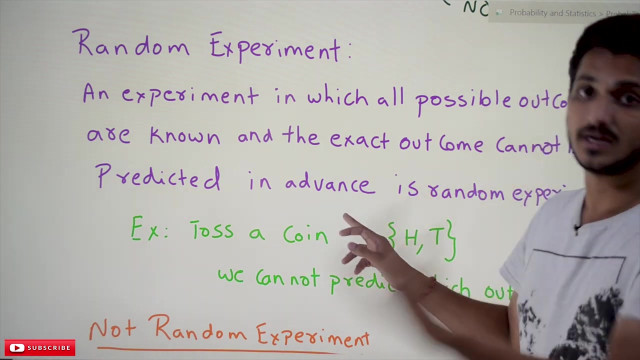 So watch carefully An experiment in which all possible outcomes are known, We know when we do the experiment, we know what outcomes it is going to get, And the exact outcome cannot be predicted in advance. That is what random experiment means: The exact output cannot be predicted in advance. 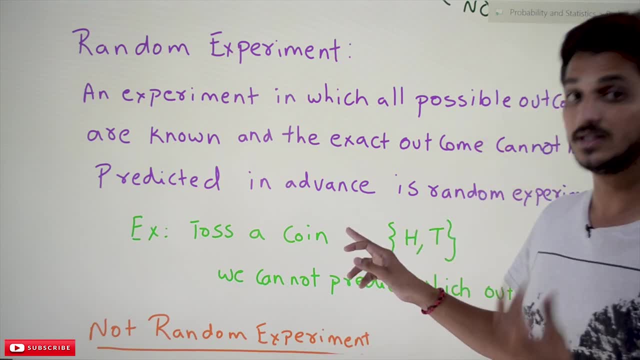 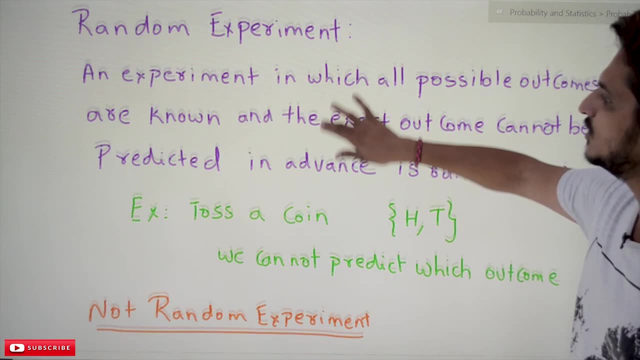 We know all the possible outcomes, But the exact outcome cannot be predicted in advance. That is what random experiment means. Anyhow, with example, you are going to understand better If you toss a coin, what is the possible outcomes that you are going to get. 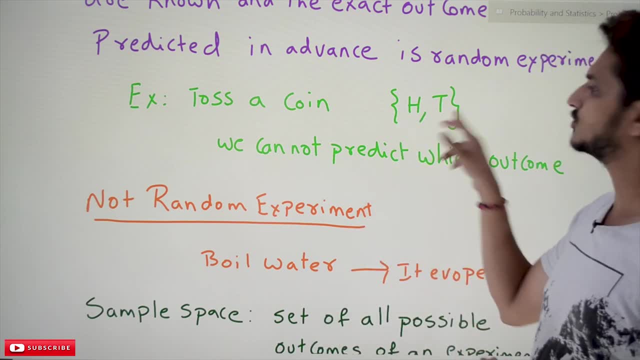 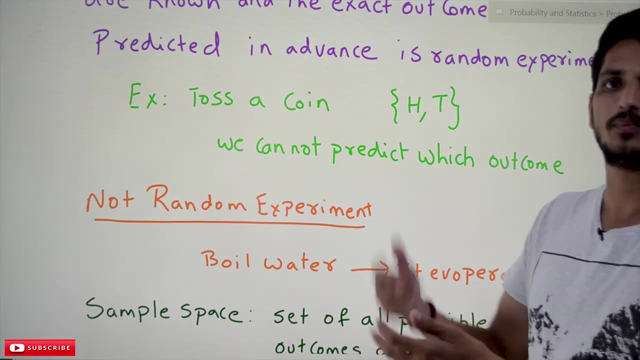 When you toss a coin. it may show up head, it may show up tail, But what is the exact output that it is going to come? We don't know. It may show up head, it may show up tail. These are the possible outcomes. 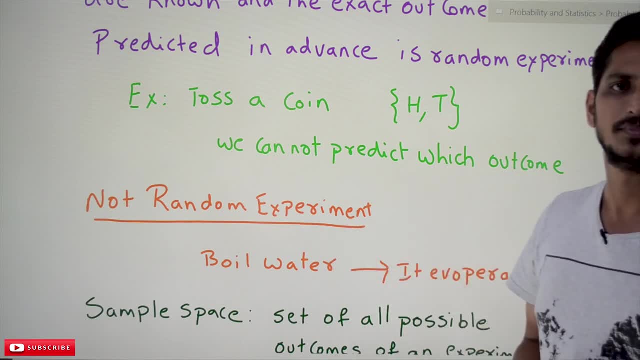 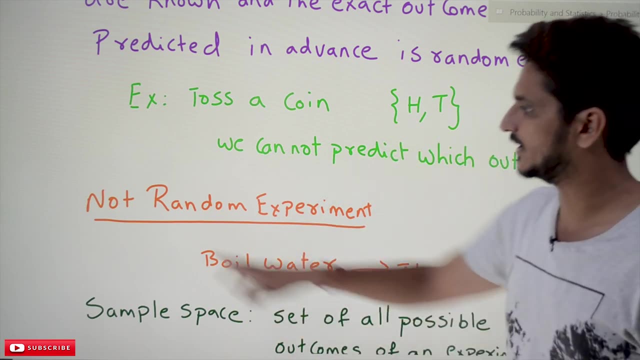 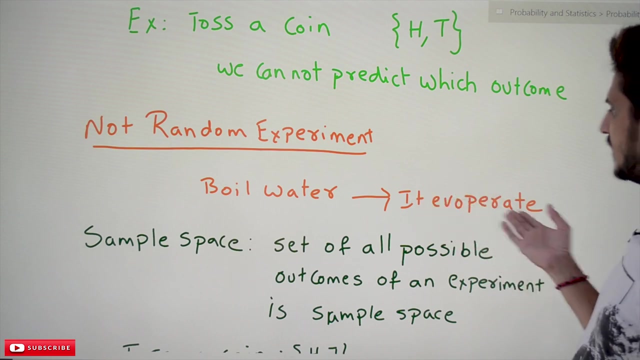 We cannot predict which outcome it is going to come. That is what random experiment means. So let's try to understand one more example, which is not a random experiment. If you boil water, what is going to happen? Water will evaporate. You know the output. 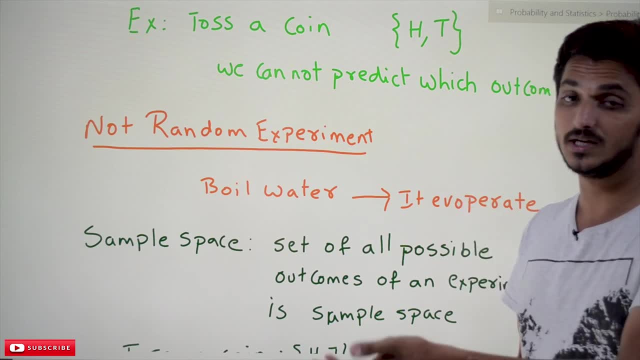 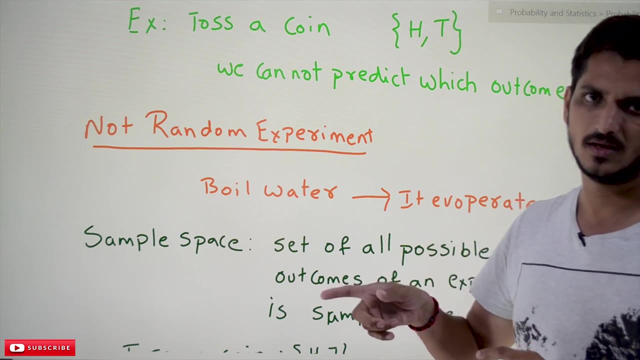 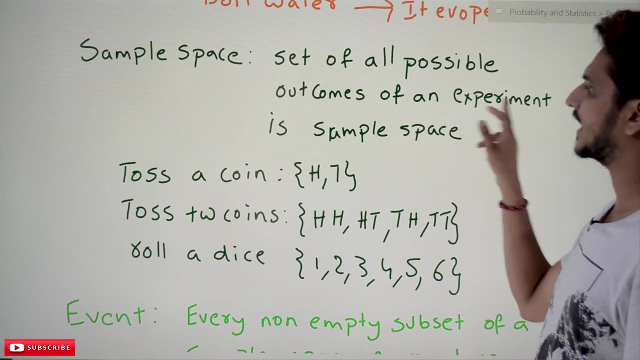 It is easy to predict the output In random experiment. you cannot predict the output. That is what the difference between experiment and random experiment. Now, coming to that sample space Set of all possible outcomes of an experiment is sample space. What are all the possible outcomes that you are going to get in a random experiment? 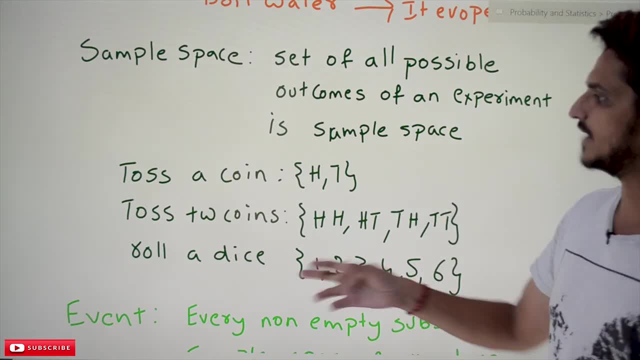 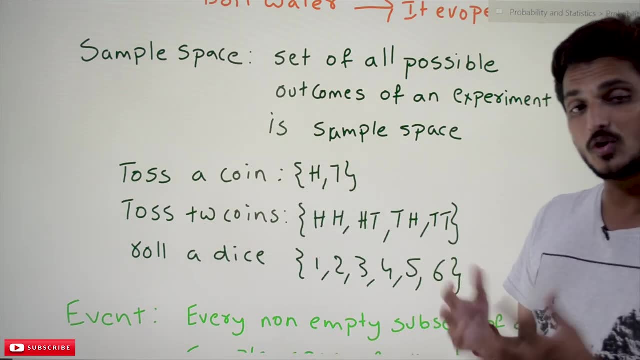 That we call it as sample space. Example: toss a coin: What is the possible outcomes that you are going to get Head tail. Toss two coins: What are the possible outcomes that you are going to get Head head. 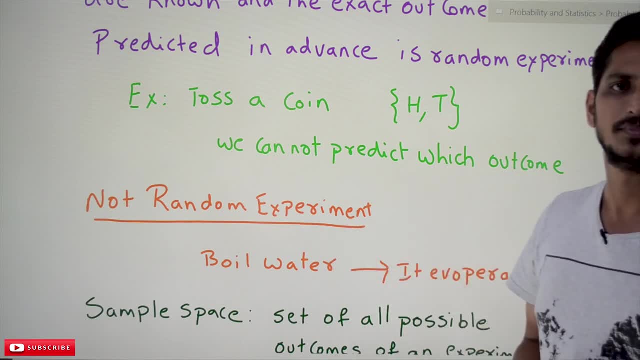 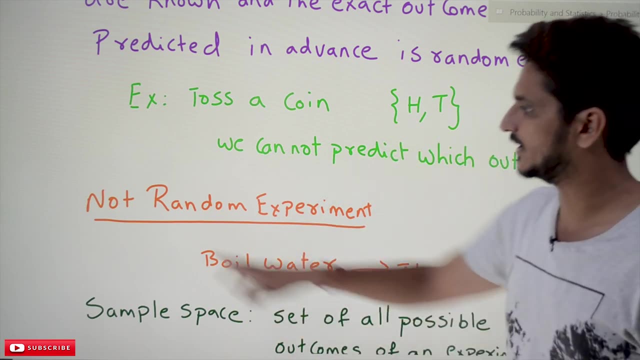 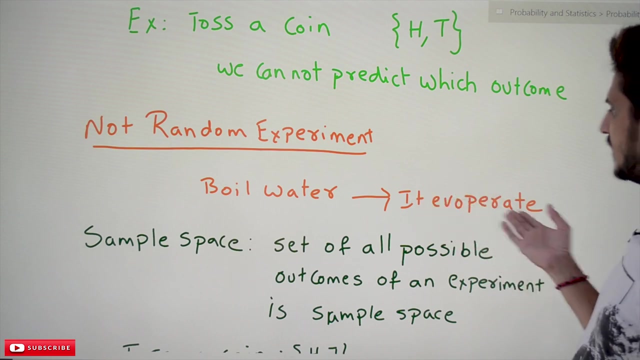 We cannot predict which outcome it is going to come. That is what random experiment means. So let's try to understand one more example, which is not a random experiment. If you boil water, what is going to happen? Water will evaporate. You know the output. 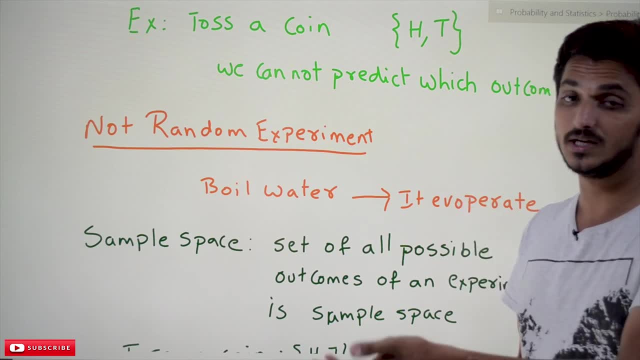 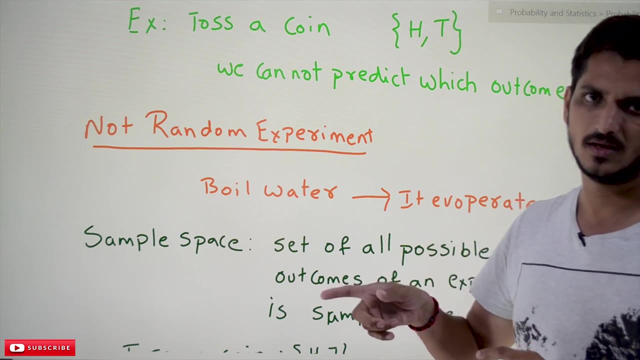 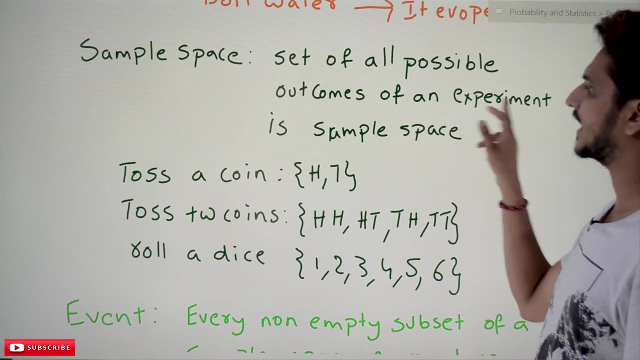 It is easy to predict the output In random experiment. you cannot predict the output. That is what the difference between experiment and random experiment. Now, coming to that sample space Set of all possible outcomes of an experiment is sample space. What are all the possible outcomes that you are going to get in a random experiment? 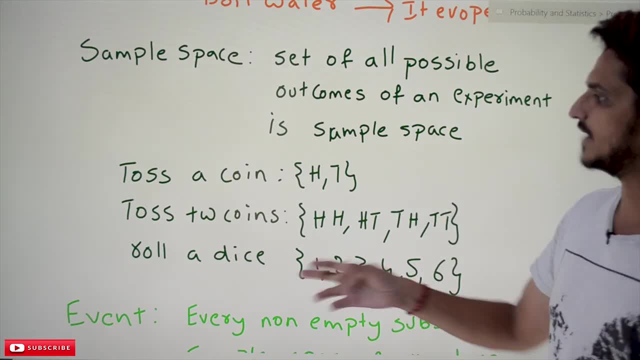 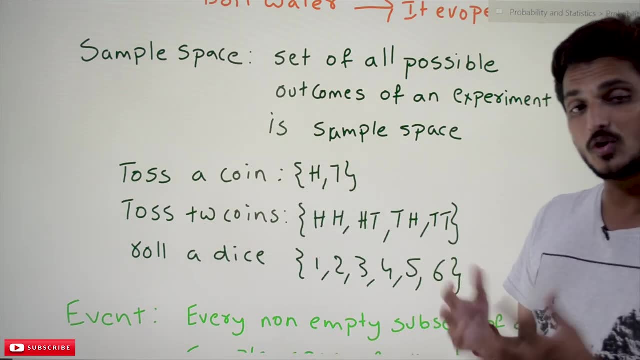 That we call it as sample space. Example: toss a coin: What is the possible outcomes that you are going to get Head tail. Toss two coins: What are the possible outcomes that you are going to get Head head. 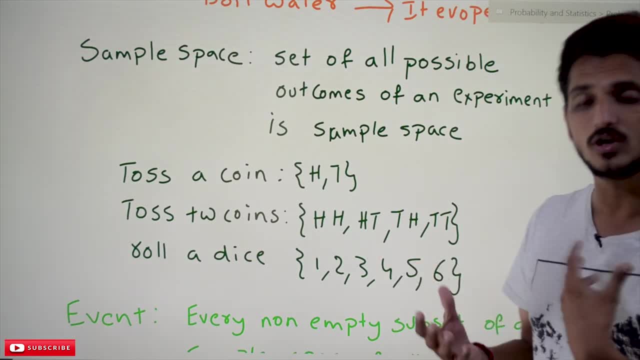 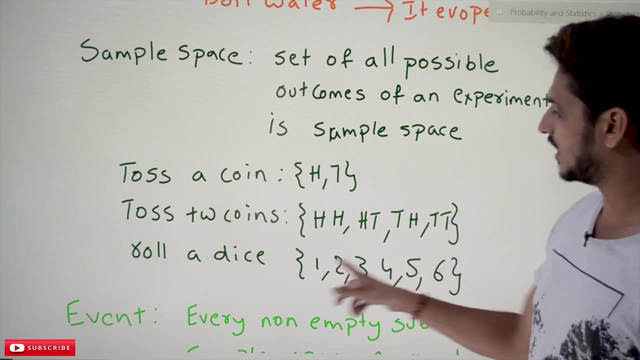 Head, tail, Tail. head, Tail, tail. These are the possible outcomes it is going to get if you toss two coins. The third one is roll a dice. What is the possible outcome? you are going to get One, two, three, four, five, six. 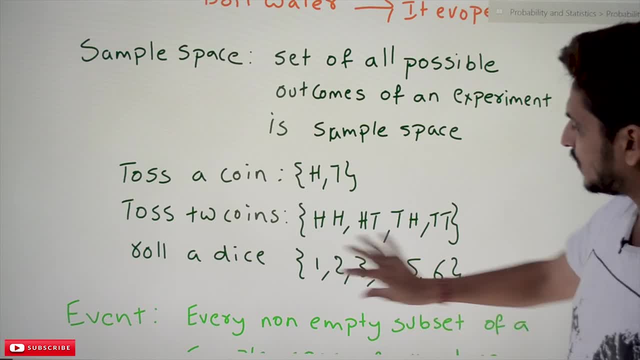 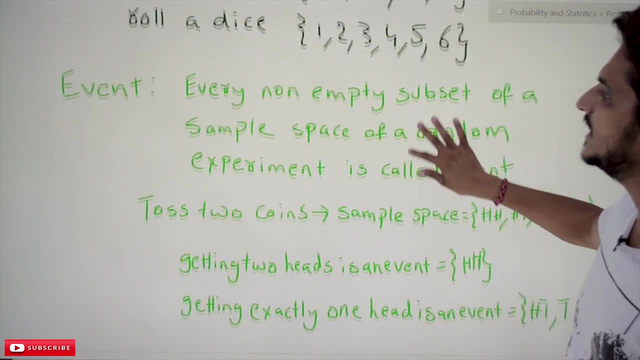 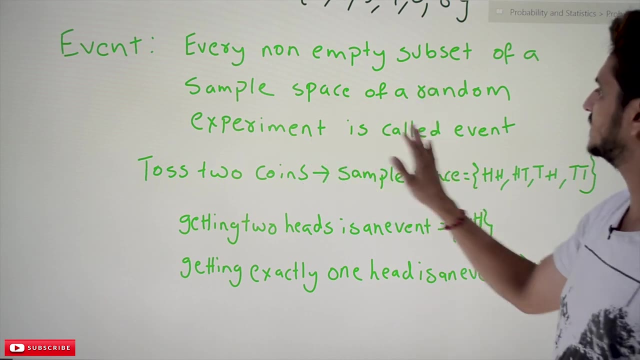 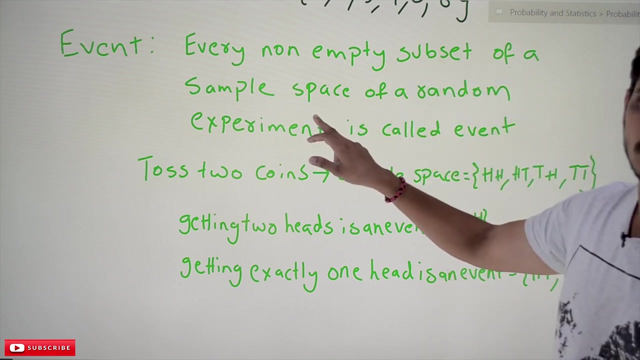 Any one you are going to get. These are all the possible outcomes. That is what we call it as sample space. Now, coming to the next definition: event. Every non-empty subset of a sample space of a random experiment is called event. So every non-empty subset of a sample space, we call it as an event. 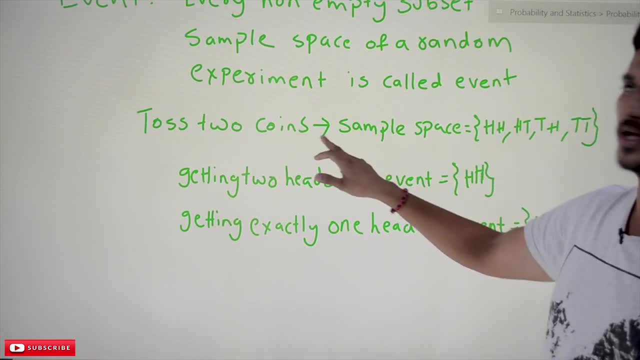 With example you will get to understand better. Toss two coins. What is the sample space? It may show up head, head. It may show up head, tail, Tail, head, Tail, tail. So, coming to that, this is what we call it as sample space. 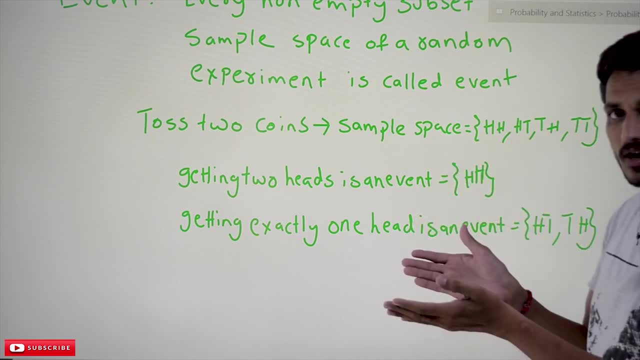 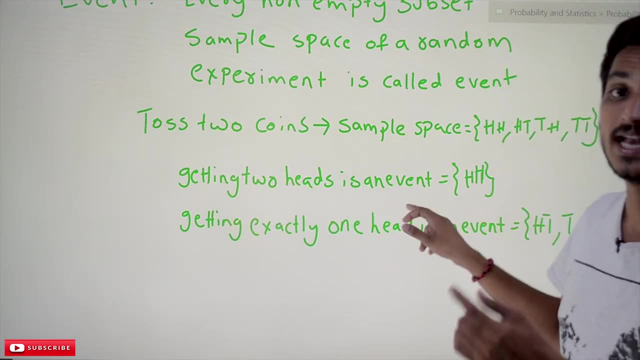 Every non-empty subset of this sample space. we call it as an event Means when you toss two coins. showing two heads is an event. So how many possibilities are there? showing two heads? One possibility, Head head, One more event. 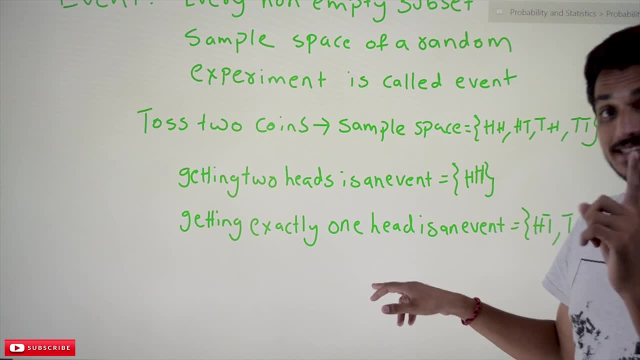 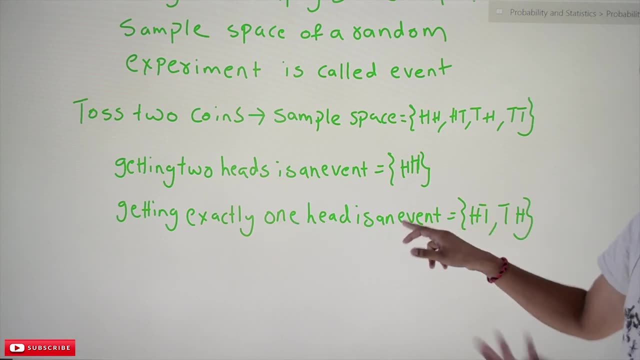 One more event: Getting exactly one head, Exactly one head. There are two possibilities showing that is an event: Exactly one head It is an event. So what are the possibilities that you are having that? showing one head on the one, exactly one head. 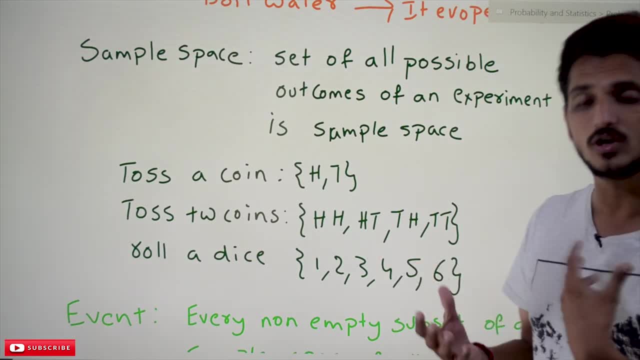 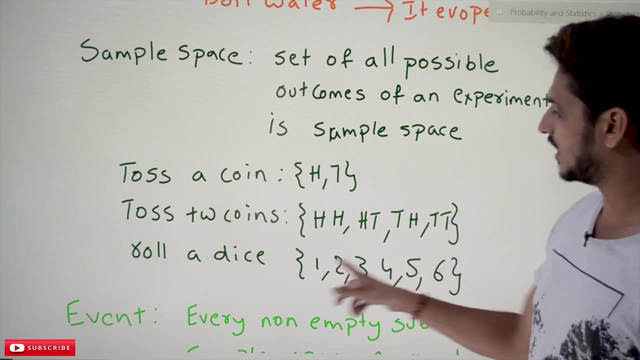 Head, tail, Tail. head, Tail, tail. These are the possible outcomes it is going to get if you toss two coins. The third one is roll a dice. What is the possible outcome? you are going to get One, two, three, four, five, six. 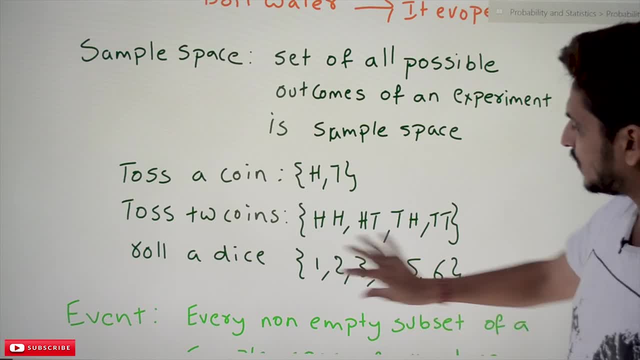 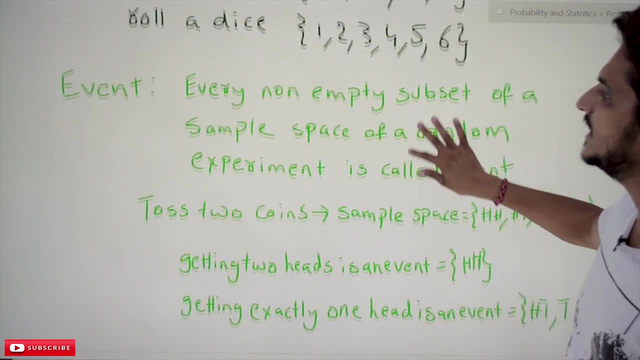 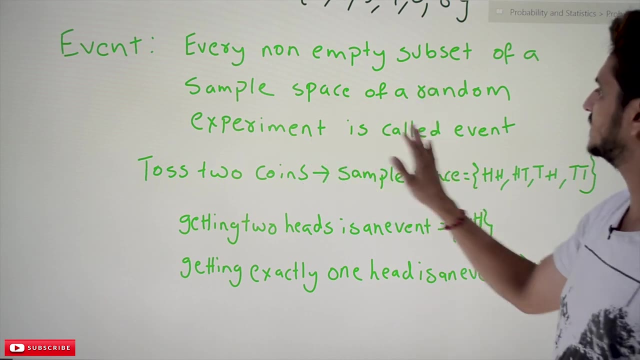 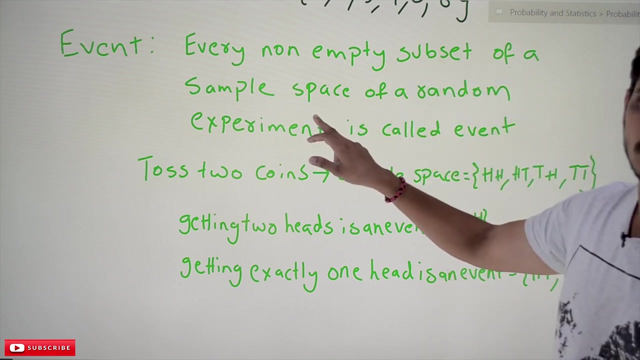 Any one you are going to get. These are all the possible outcomes. That is what we call it as sample space. Now, coming to the next definition: event. Every non-empty subset of a sample space of a random experiment is called event. So every non-empty subset of a sample space, we call it as an event. 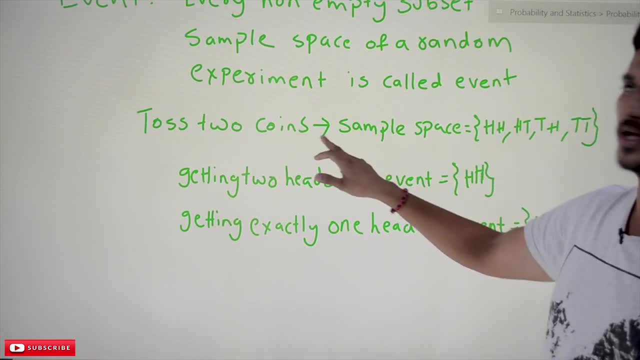 With example you will get to understand better. Toss two coins. What is the sample space? It may show up head, head. It may show up head, tail, Tail, head, Tail, tail. So, coming to that, this is what we call it as sample space. 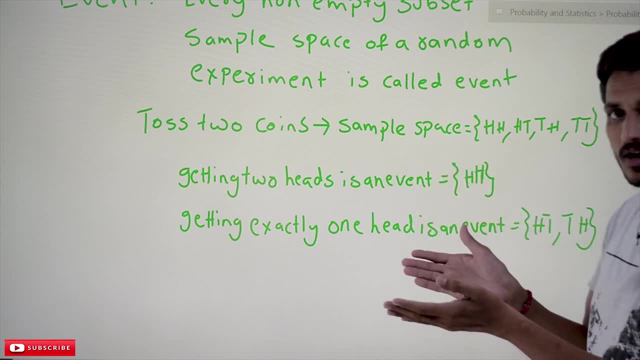 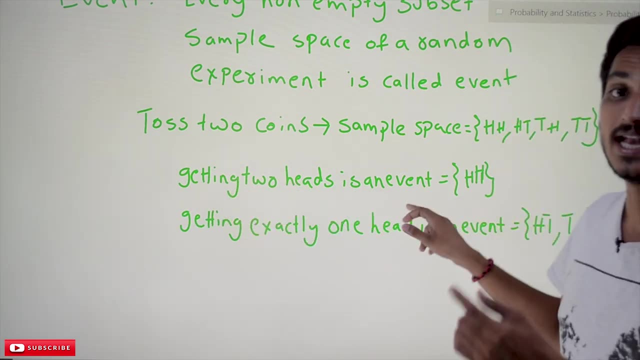 Every non-empty subset of this sample space. we call it as an event Means when you toss two coins. showing two heads is an event. So how many possibilities are there? showing two heads? One possibility, head head. One more event, one more event. 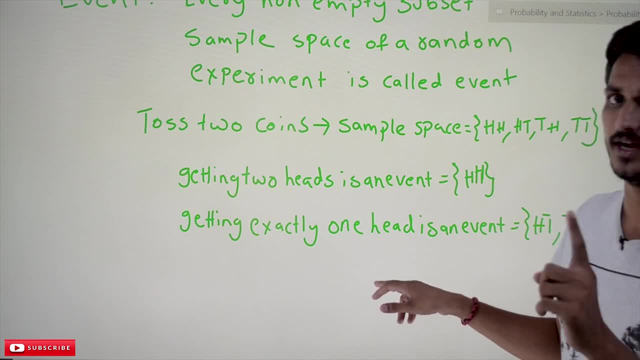 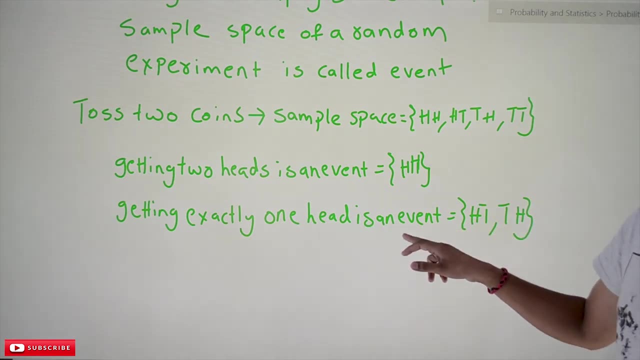 Getting exactly one head, exactly one head. There are two possibilities showing that is an event: Exactly one head, it is an event. So what are the possibilities that you are having that showing one head on the exactly one head? Either first one shows head, second one shows tail. 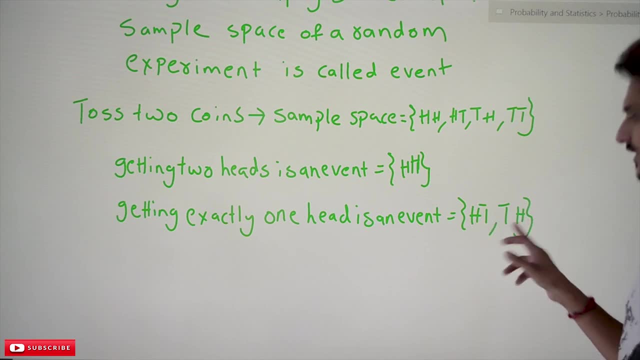 Either first one shows tail, second one shows head. These are the possible events that you are going to obtain. required event. So from the sample space, what are the possible subsets, non-empty subsets of the sample space. we call it as an event. 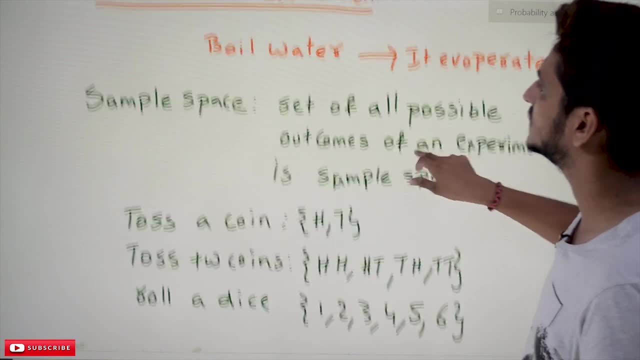 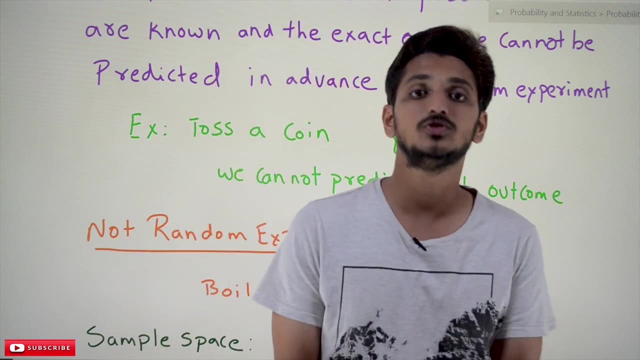 So if you understand these definitions, it is very easy to understand the remaining concepts which we are going to discuss in our coming classes. Hope you understand the concept. If you have any questions regarding the concept, please post your questions in the comment section below. 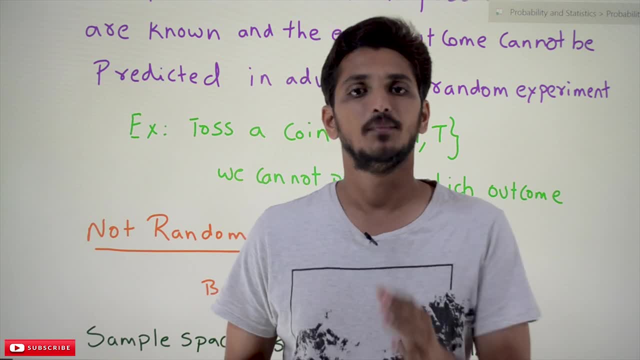 Thanks for watching. If you haven't subscribed to our channel, please subscribe to our channel and press bell icon for the latest updates. Thank you.